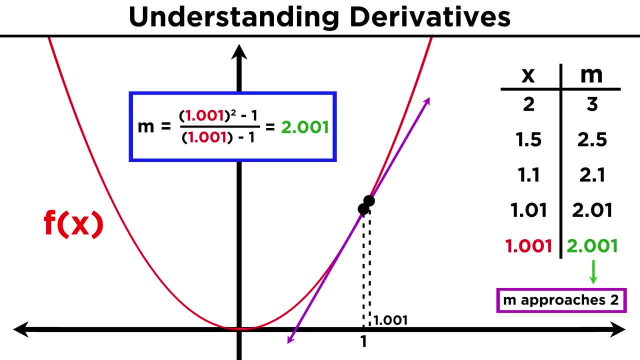 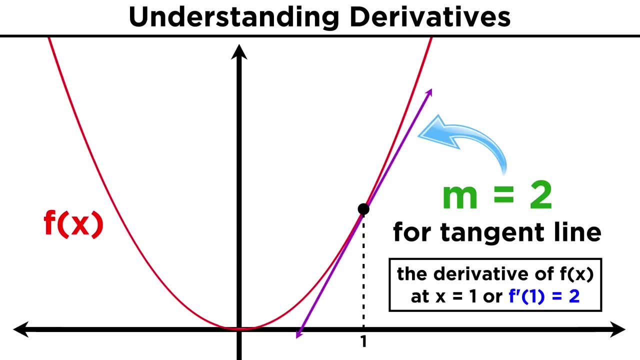 When we first introduced differentiation, we looked at a method for calculating the slope of a tangent line. By using this method of exhaustion, we were performing differentiation and in doing so, we found the derivative of this function at this point. This derivative was defined to be the slope of the tangent line at this point and the 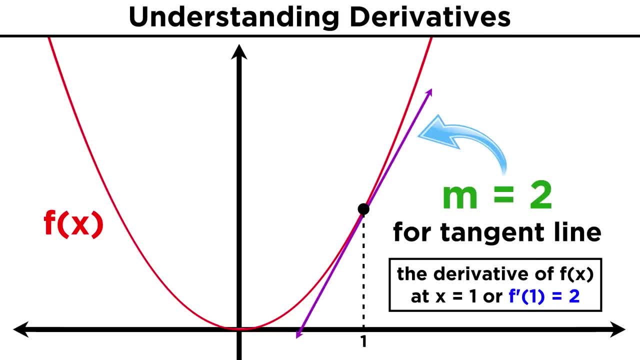 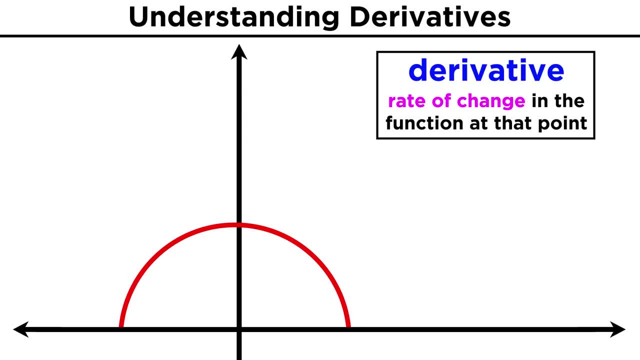 slope of the line was derived from the function. The derivative of a function tells us about the. the derivative of a function tells us about the rate of change in that function at a particular input value. If a function is increasing at a particular point, its derivative is positive at that. 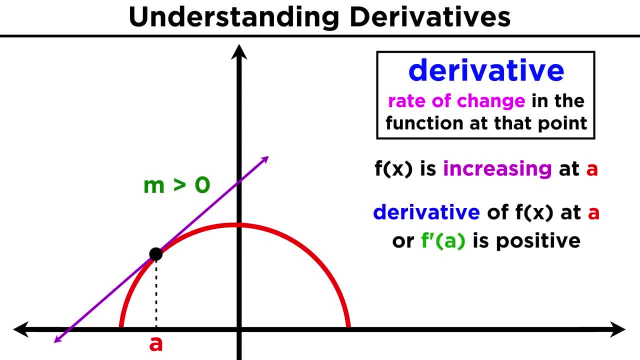 point, which is just a fancy way of saying that the slope of its tangent line is positive at that point. If a function is decreasing at a particular point, its derivative is negative at that point and the slope of its tangent line will be negative. 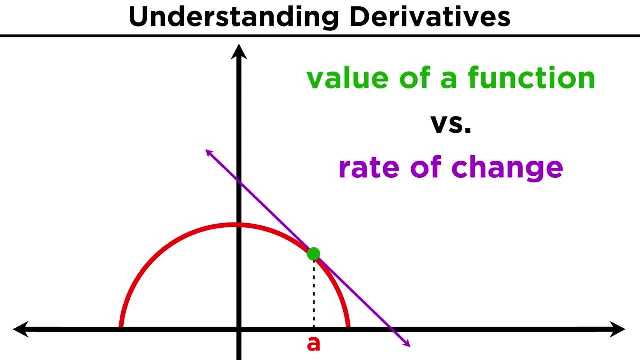 Let's take a moment to note something here. It is crucial that we mentally separate the value of a function at some point from the change in that function at that point. If, examining position and speed, we could be located at the origin, meaning our position. 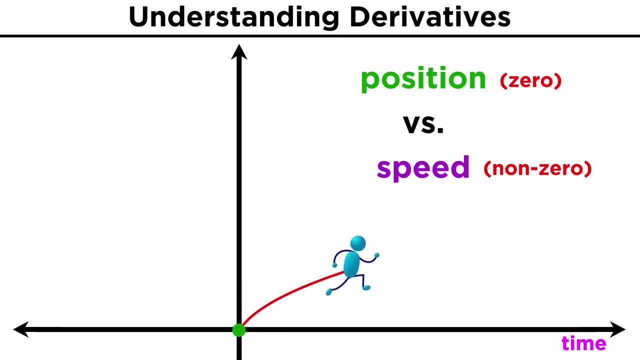 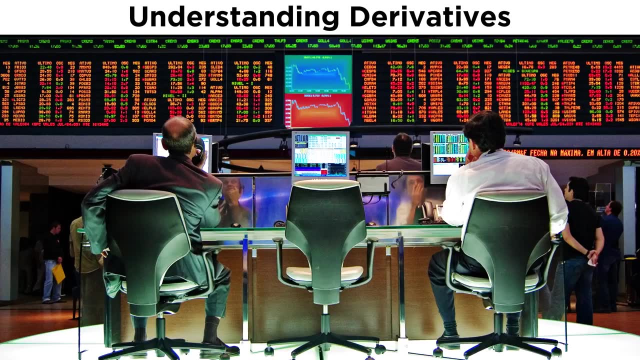 is zero, but with non-zero speed, meaning we aren't standing there but just passing by. Or we could be at some other non-zero location, but standing still with zero speed. We can also think of stock prices. These can be high or low, but their values are typically unrelated to their rate of change. 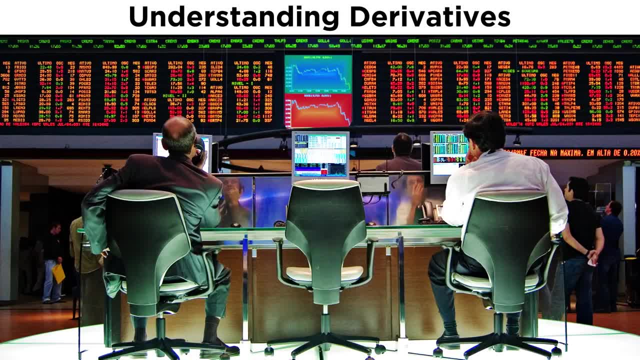 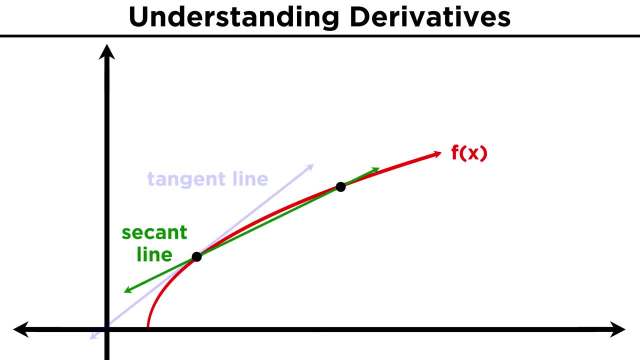 They could continue to climb or plummet at any moment. Now, looking at the tangent line again, let's formalize this a little bit more. Remember that our method involved choosing a second point on the curve. We can give the first point the coordinates A, F of A. 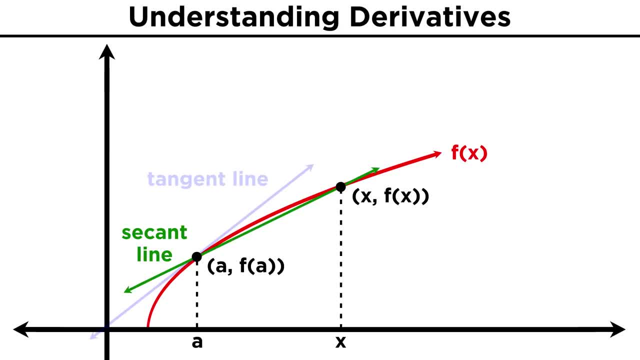 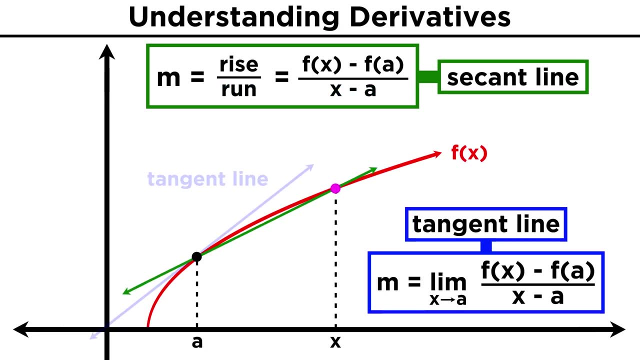 And the second point can be X, F of X. As we said, the slope of this line, which we can call the secant line, is rise over run, so F of X minus F of A, over X minus A. Then we can allow point X to approach point A, and we said that the slope of the tangent 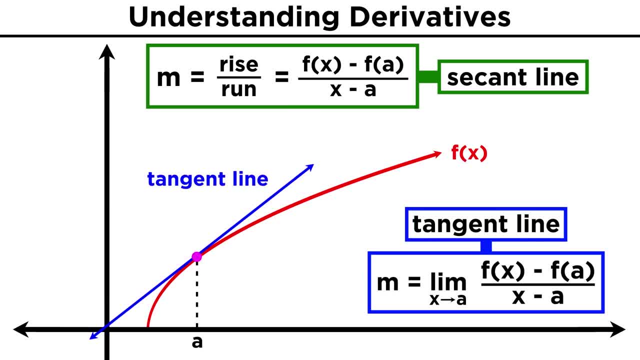 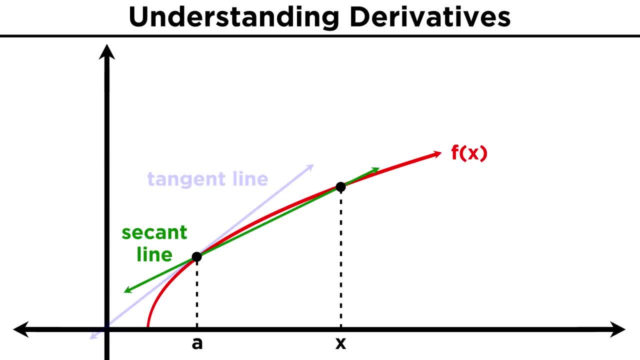 line will be the slope of this secant line in the limit of X approaching A. We can express this another way with the second point, in terms of the first, by saying that X is equal to A plus some other quantity, H. So H is the distance in the X direction. 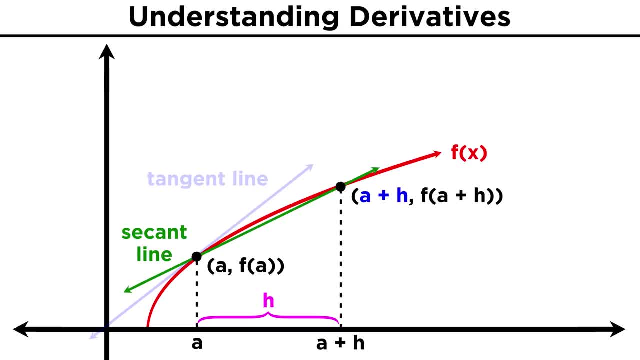 from the first point to the next. That means this second point has the X coordinate A plus H and the Y coordinate F of A plus H. Now to get rise over run, we find F of A plus H minus F of A over H. 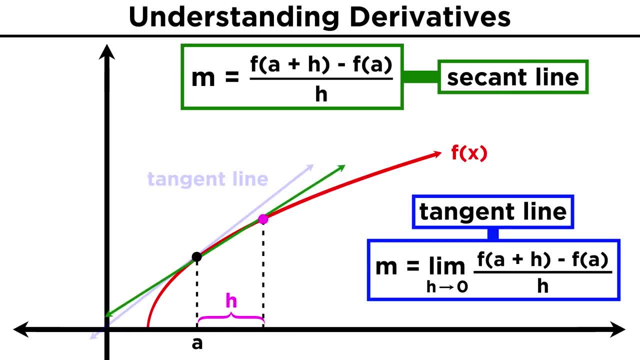 This time, the slope of the tangent line is the limit of this expression, as H approaches zero, meaning the distance between the two points becomes zero and the points become one. What we must understand is that we can just as easily calculate the slope of the tangent. 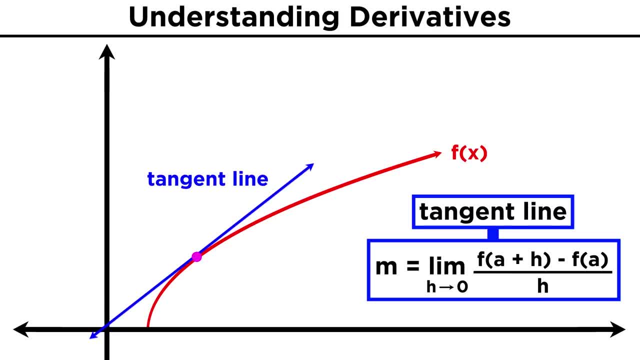 line, which is the limit of this expression. as H approaches zero, meaning the distance between the two points becomes zero and the points become one. We can just as easily refer to this value as the slope, not just of the tangent line, but the slope of the curve itself at this precise point. 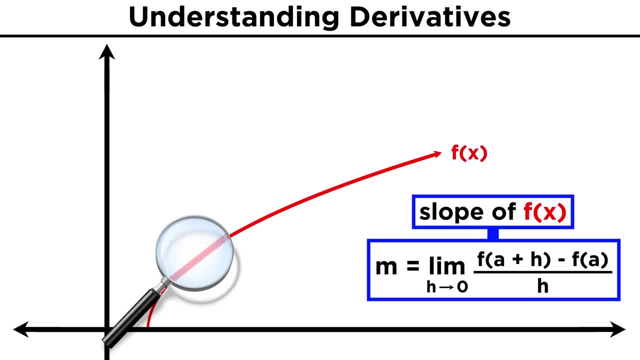 If we were to zoom into the curve at this point closer and closer, it would eventually resemble a line with this slope And, in fact, combining this knowledge with this expression will give us a better understanding of the definition of a derivative. The derivative of some function. F at some interval is a derivative of some function. 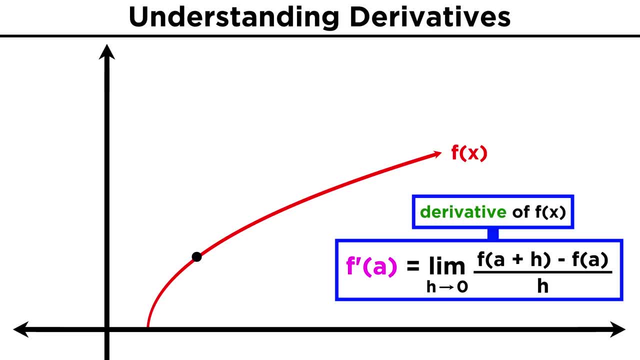 F at some interval, The derivative of some function F at some interval is a derivative of some function F. The sum of a function's input value, A, which we can represent as F prime of A, is precisely this expression we just described. 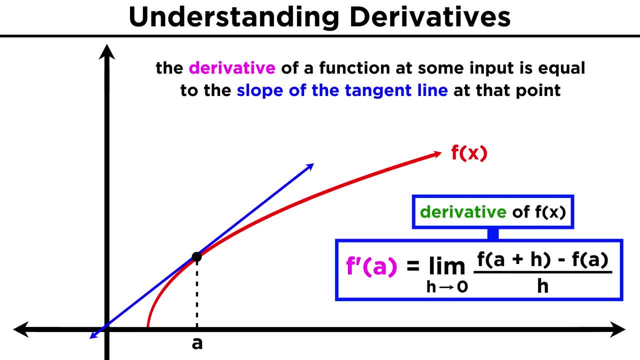 So, to put it in words, the derivative of a function at some input is equal to the slope of the tangent line at that point. Identically, the derivative of a function at some input is equal to the rate of change of the function at that point. 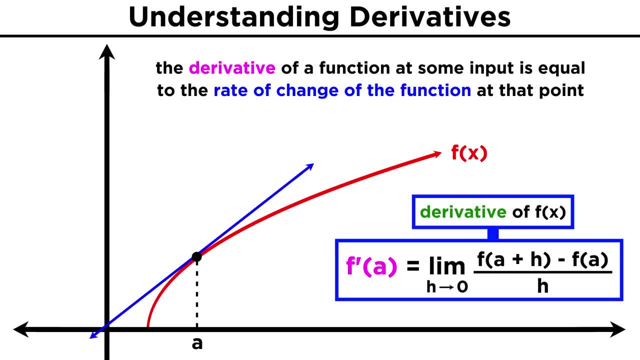 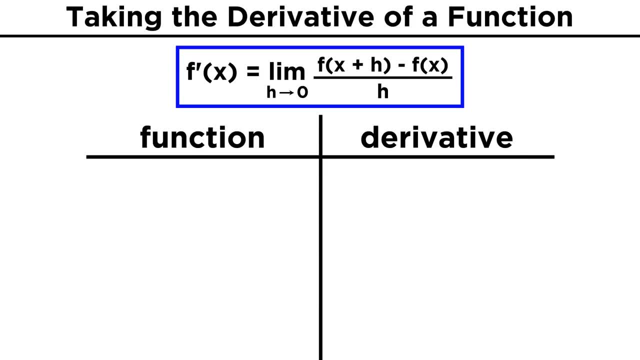 These are two ways of saying the happy ending. precisely the same thing, and that thing is the derivative of the function. Let's use this expression to take the derivative of some different functions. Let's start with something easy. how about some constant function like f of x equals? 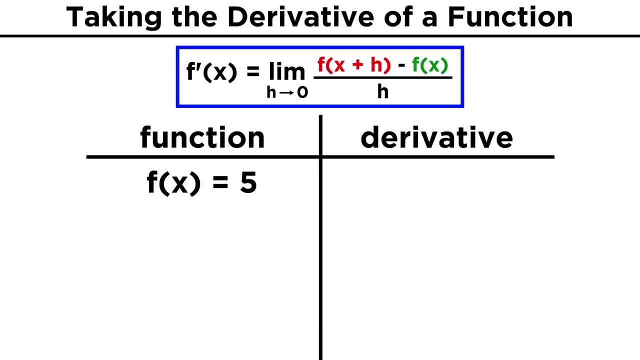 five. If we take the derivative of this, when we go to plug in values for f of x plus h and f of x, these will both be five because no matter what point on the function we are talking about, it's equal to five. 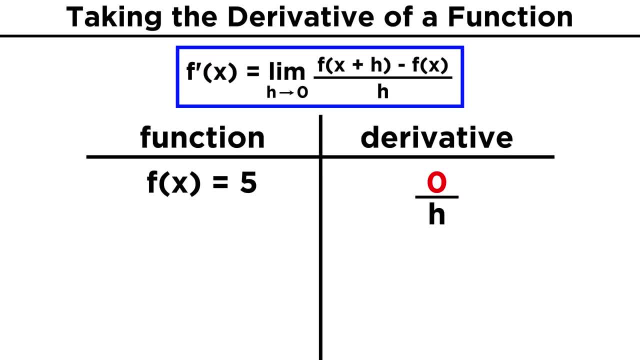 Five minus five is zero. so as h approaches zero, f prime of x will become zero. This makes sense as the rate of change anywhere on this function is zero, because the value of the function never changes. So let's make a note that when we take the derivative of a constant, any constant- it 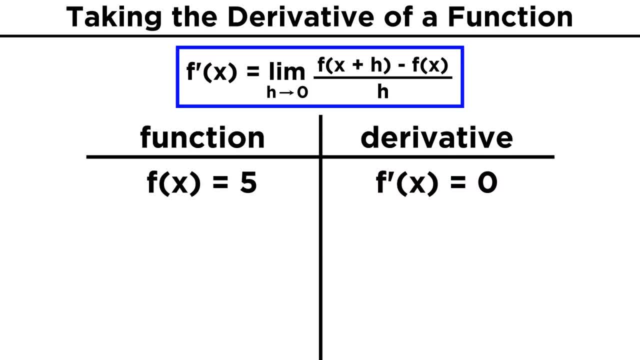 will always be zero. This should be reassuring, Because it means that our precise math is aligning with the intuitive idea we wanted it to reflect. Now let's try the function. f of x equals x. If we try to find the derivative of this for f of x plus h, we get x plus h, and for: 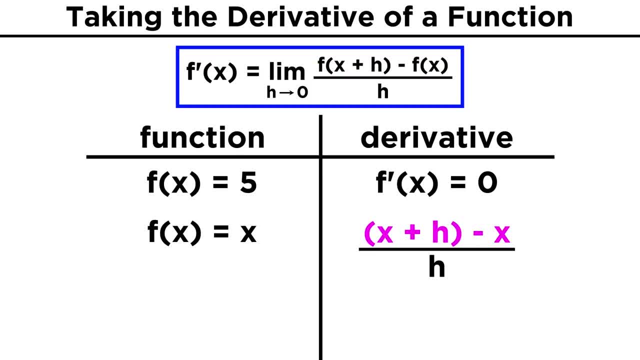 f of x, we get x. So x plus h minus x means the x's cancel, which gives us h and h over h is one, So the derivative of x is zero, Then x is one. Now let's try x squared. 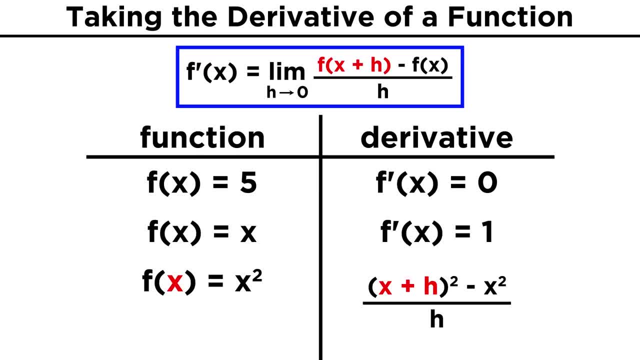 Up top. remember that we are plugging x plus h into the function first. so we have x plus h, quantity squared minus the function itself, or x squared. Now we have to FOIL this first term on the top and we get x squared plus two x h plus. 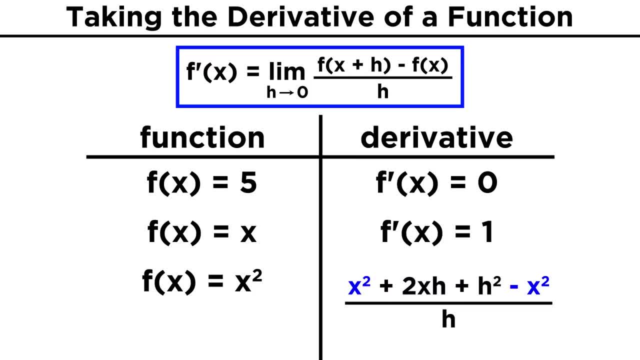 h squared minus the x squared, And that leaves zero to zero. when x is squared, Professor Pirini belts us with two X H plus H squared. Dividing both terms on top by the H on the bottom, we get two X plus H. and when H goes, 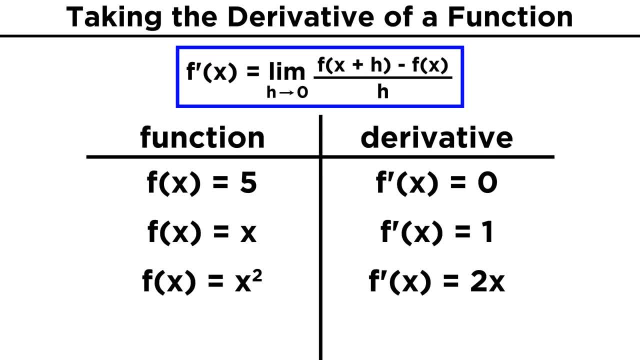 to zero. that leaves us with two X. So the derivative of X squared is two X. Let's do one more: X cubed. Now we have X plus H, quantity cubed, minus X cubed. We should know how to cube this binomial by foiling two of them and then multiplying.